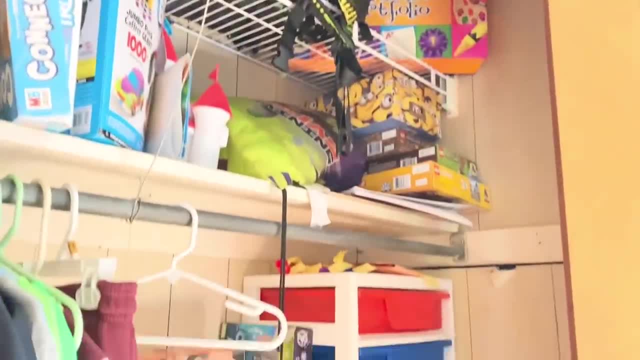 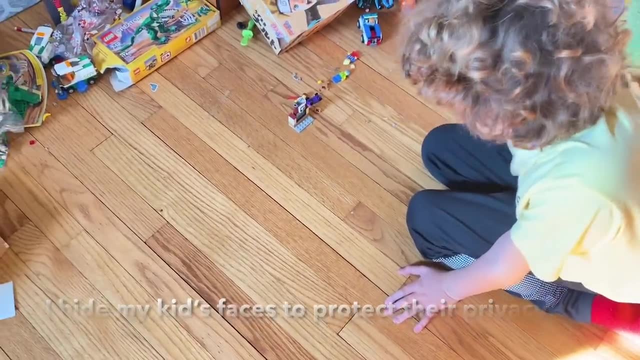 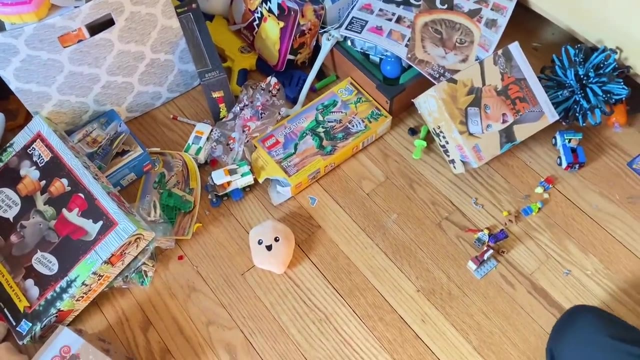 But again, this is just part of the process. But again, we're encouraging those organization behaviors. now, Where do you wanna start first? Right here, Right here. And what do you wanna do with that Lego box? What are we gonna do with it? 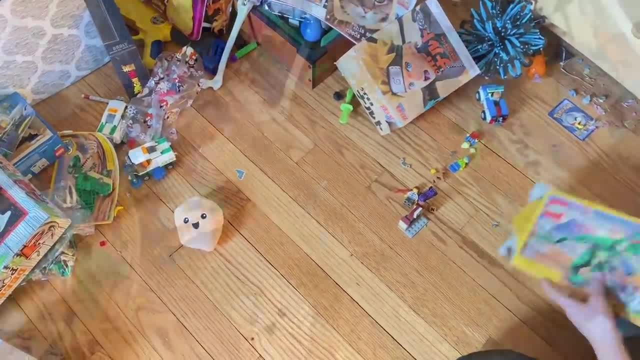 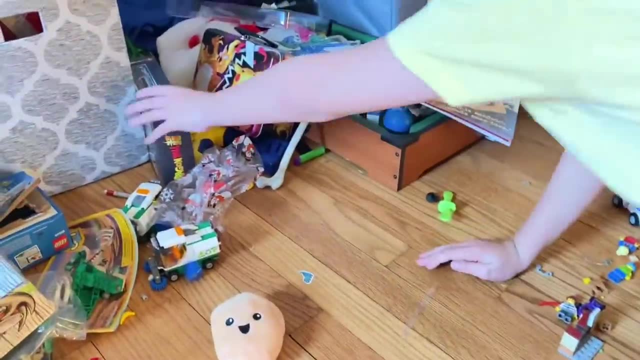 Throw it out. That's right, we're gonna throw it out. We don't need that, no-mo. What else is next? You wanna throw that out? All right. what else are you gonna throw out? Oh, empty box, right. 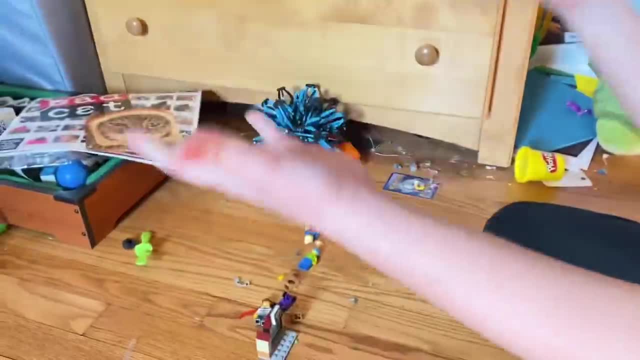 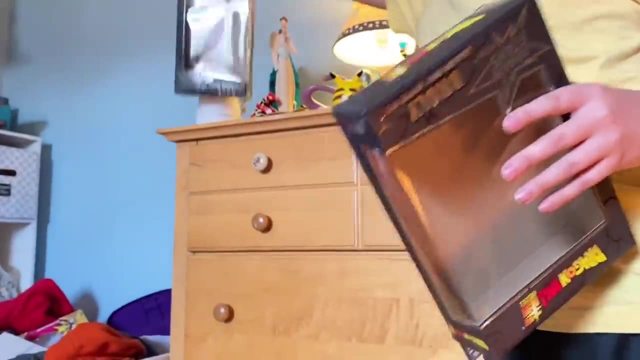 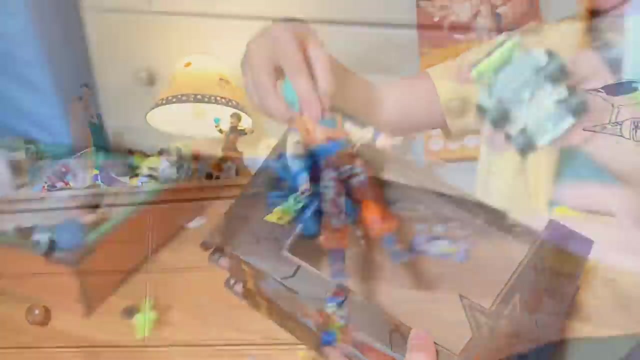 Yeah, You don't need that anymore. Where is he? That's him. You don't need the box, right? No, oh, and you don't need that box either. But you got that for Christmas, right, And you already, oh, yeah. 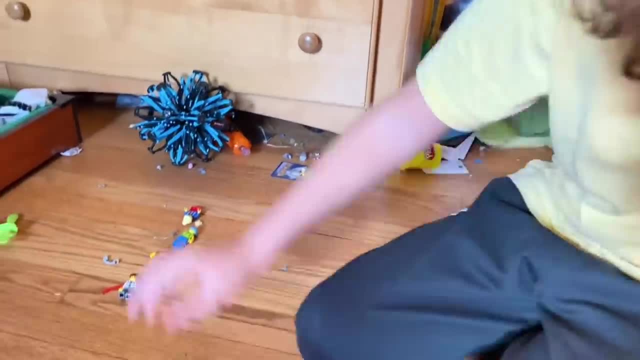 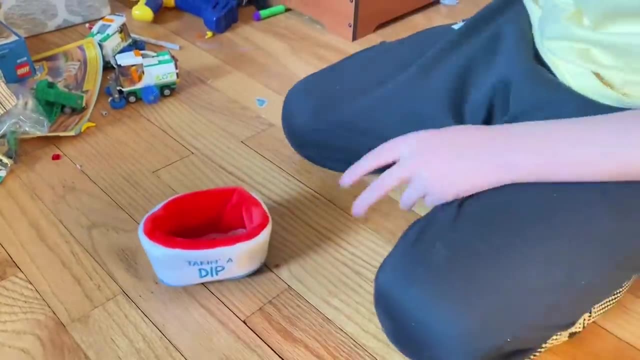 I think you're keeping your Legos. huh Yeah, you're gonna keep. oh okay, That's part of the keep pile. huh Yeah, that goes in there. Oh, there's my idea, I know, All right, so that's a keep. 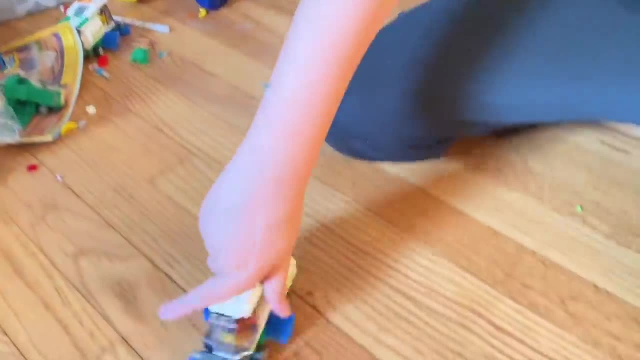 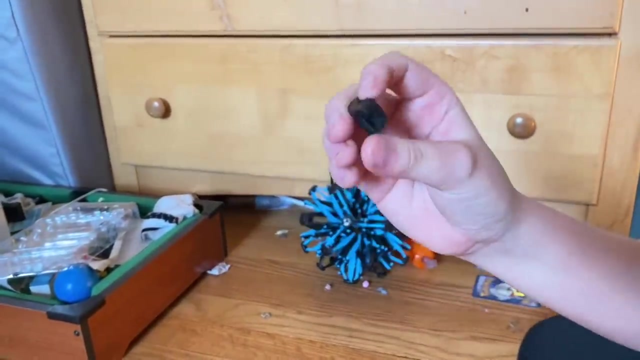 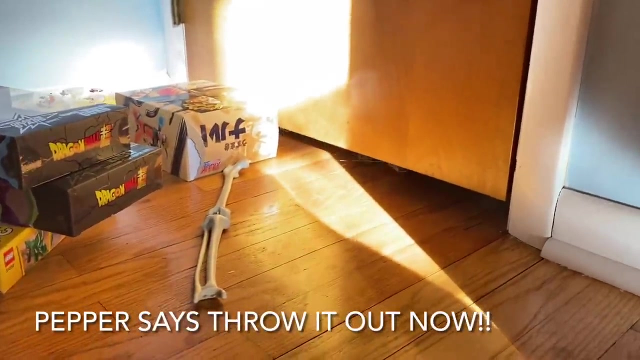 because that was that Nugget plushie. Of course that's a keep. He's cleaning it. He is cleaning it. What is that? I don't know. Toss it Like this. There's a little interruption here. What are you doing? 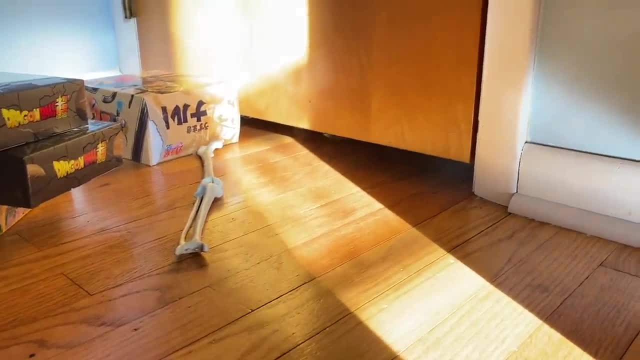 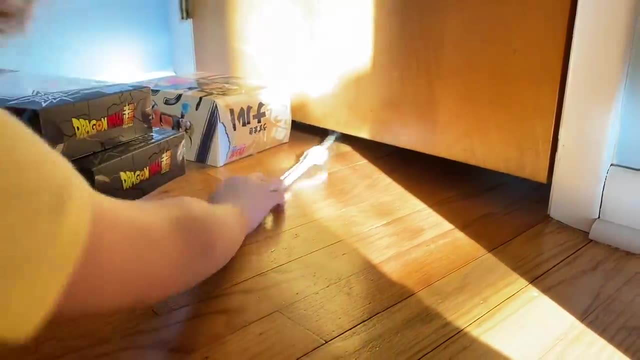 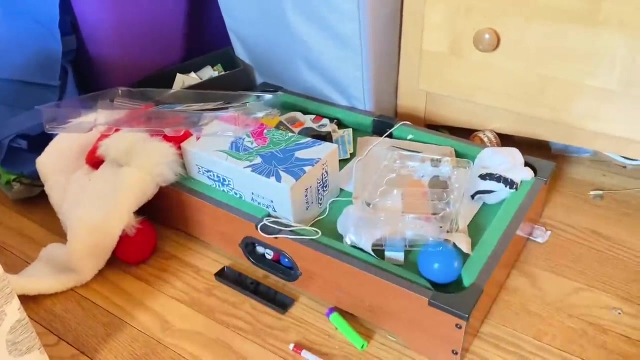 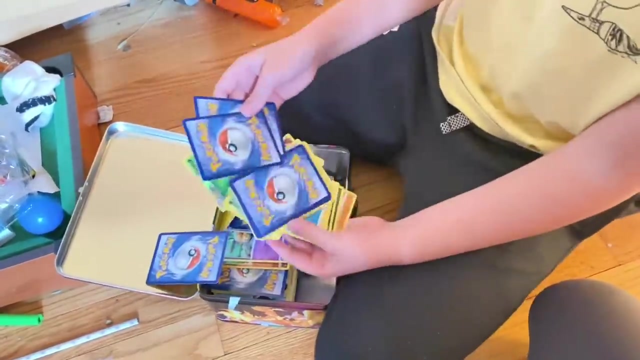 We gotta get back to our video, man, I feel it. And after our little interruption we got back to work, where Tyler was deciding what he wants to keep and what he wants to let go of. And, of course, these series with my children are probably one of the most important ones in my heart. 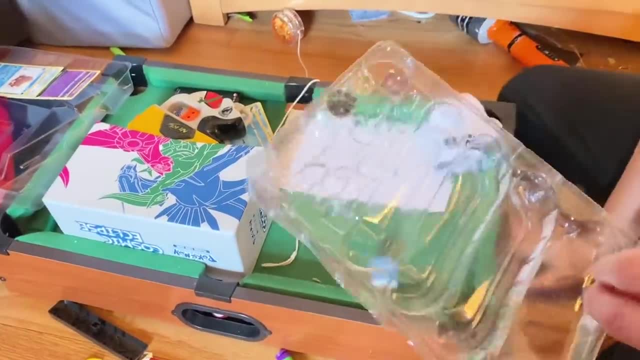 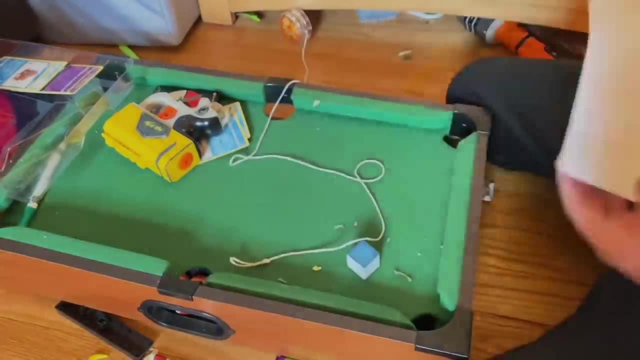 As a parent, you always want your kids to have a better life than you did, and you don't want to share the same struggles either, And I know that hoarding disorder can get passed down generation to generation. There are genetics and learned behaviors. 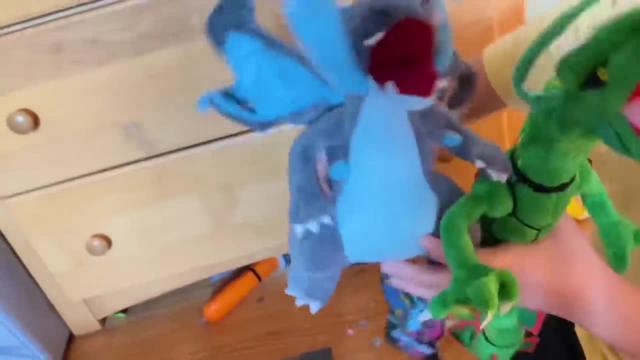 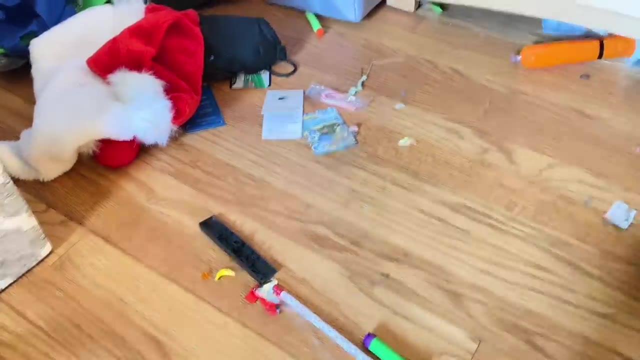 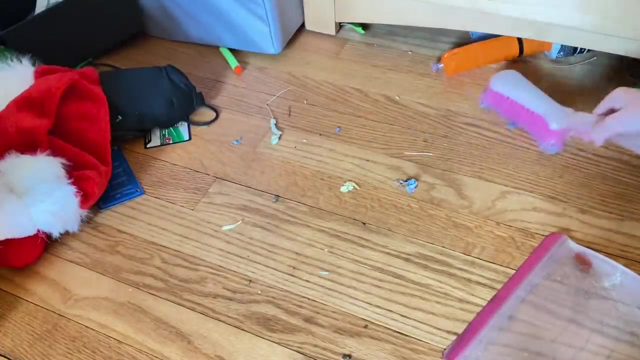 And since the boys have grown up with this- only knowing hoarding and a packed room and house- I don't want that to become their normal. I want them to learn the strategies of cleaning and organizing. And I already can tell that with Brandon he didn't develop it, He doesn't want. 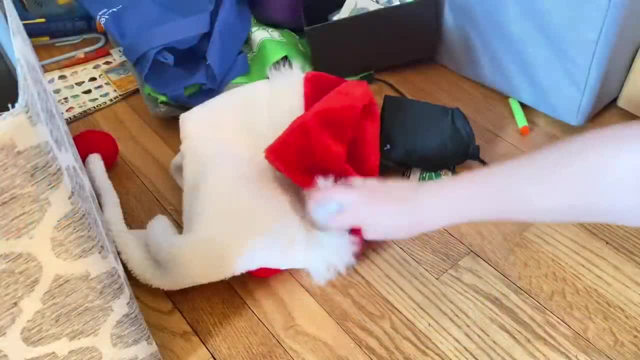 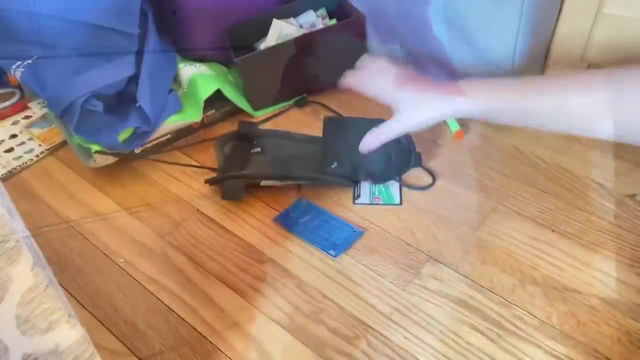 that messy room. He wants the neat and tidy room where I can tell where Tyler is having a lot more fun with his stuff, And of course a lot of that has to do with his age too, So I'm not going to look too deeply in it, other than to continue developing. 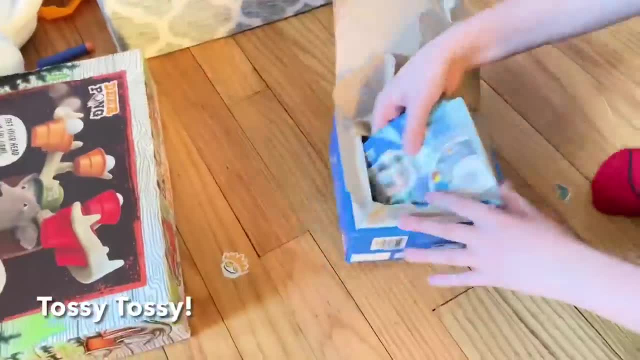 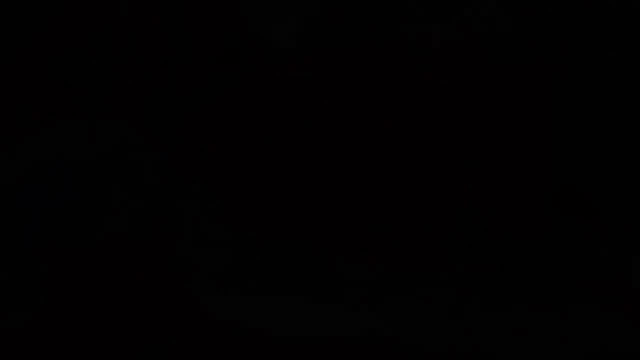 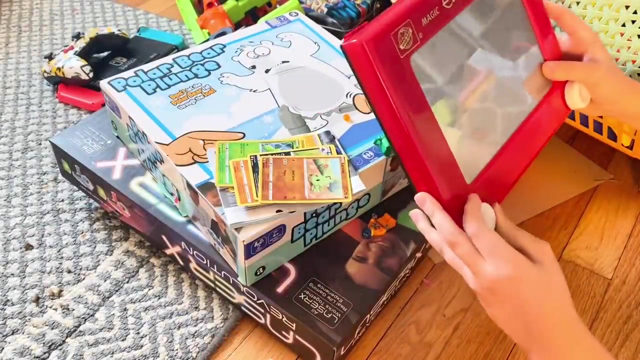 SEози Calzada. Non Déveloping Decluttering Skills, Continuing to want that desire to have a neat and tidy room And that messes and things don't create security. That was how I developed my hoarding disorder, Because I found security in all my toys and my plushies and my items. 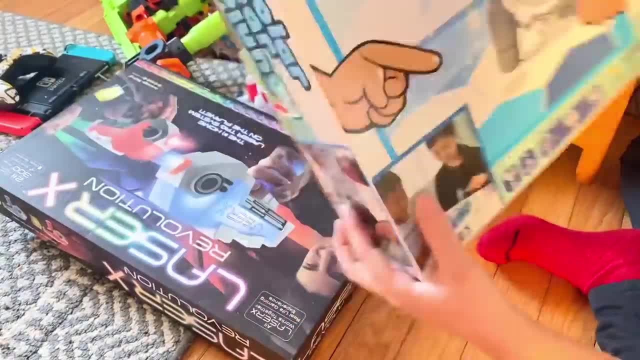 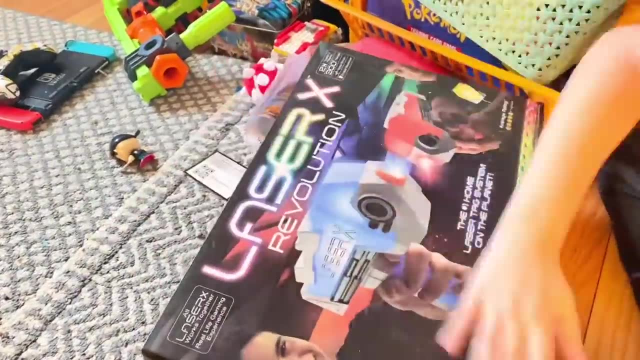 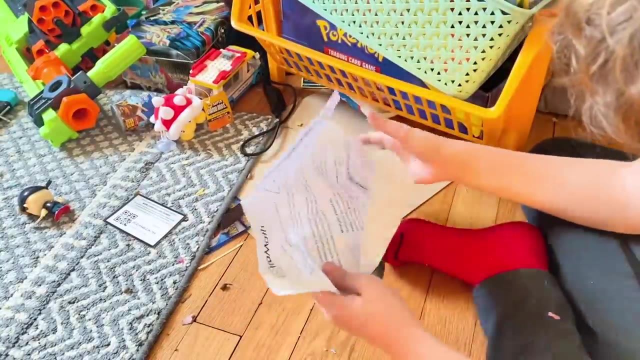 to escape being bullied in middle school. The kids were so mean to me, But at home all of my things didn't judge me, All of them didn't. SEози Calzada, call me awful, awful, disgusting names, or push me. I felt loved and security there. 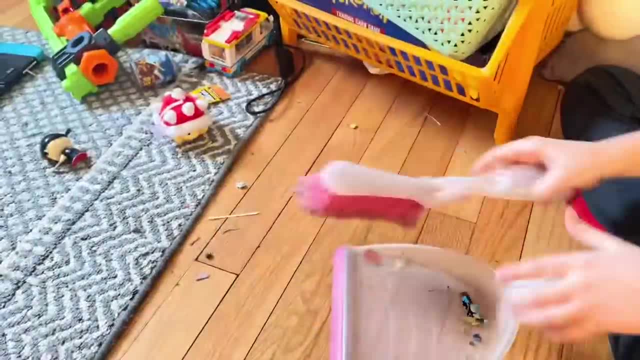 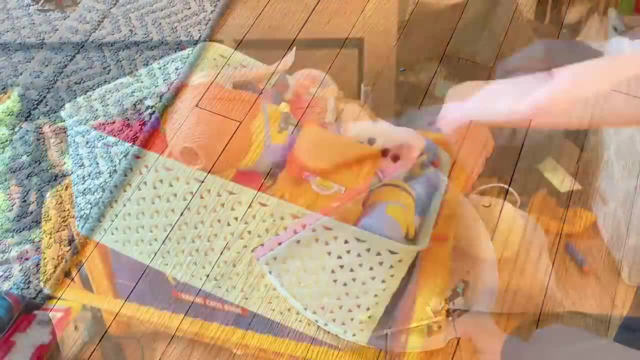 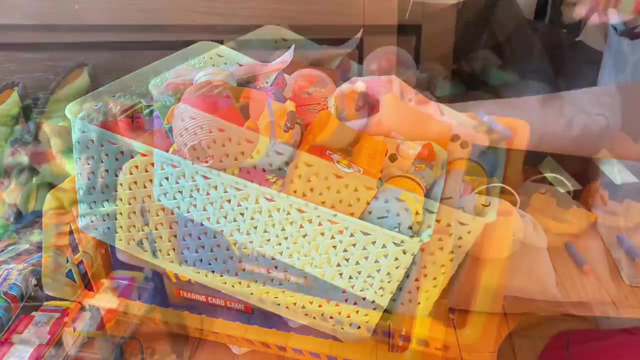 And all the while, my mom had no idea that that was developing within me. My parents had no idea that I was being bullied in school and developing hoarding behaviors to cope with all of that. because I hid it. I hid it from them And this is why these decluttering series with my boys. 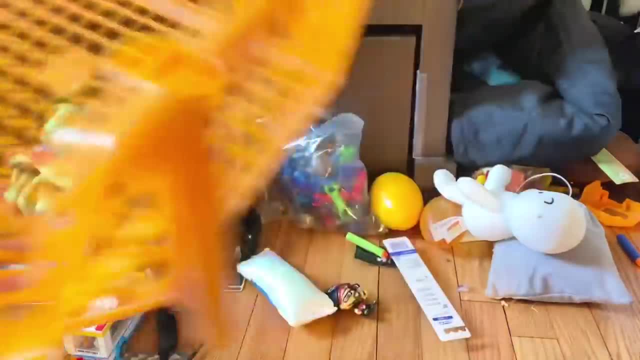 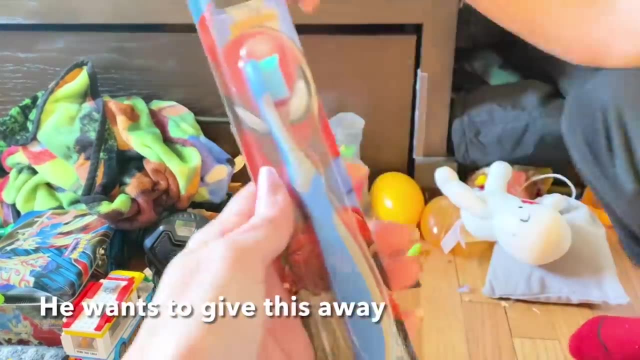 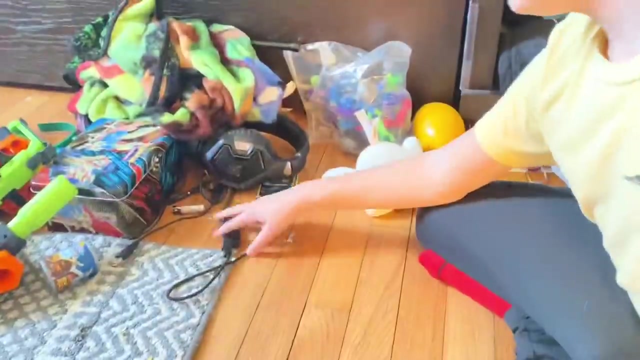 is so important to my heart and so therapeutic in my healing journey. Seeing them have the desire to want to clean their room out so that it's clean and organized is just reinforcing that 12-year-old girl inside of me who still has that need to hoard sometimes. that it's okay. 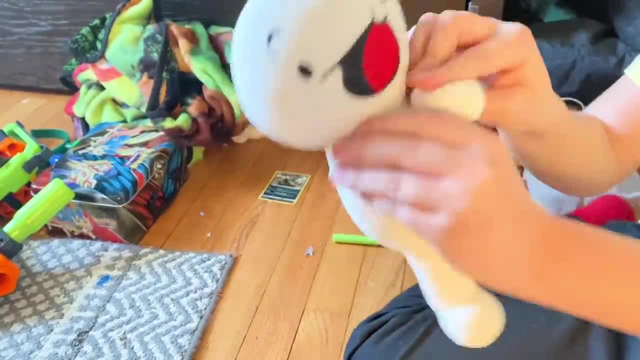 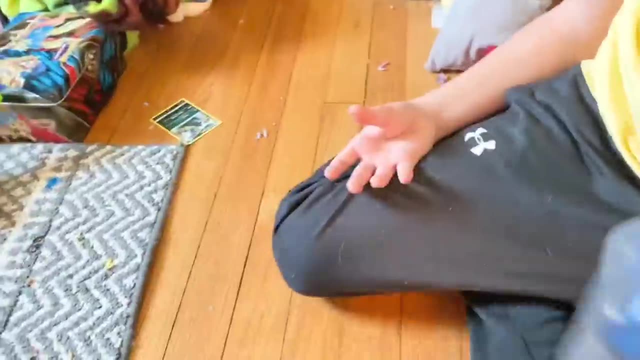 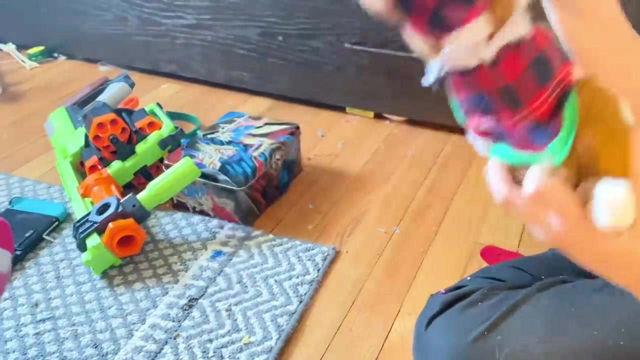 It's okay to let go of the items. It doesn't determine our self-worth. We can let it go and still have a happy and productive life. That is the message that I want my children to know, myself know, and especially all of you who might be struggling with. 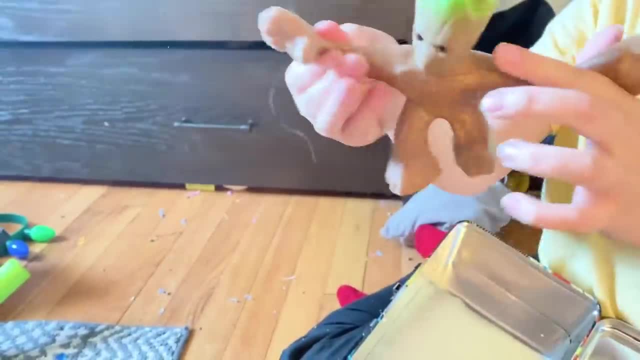 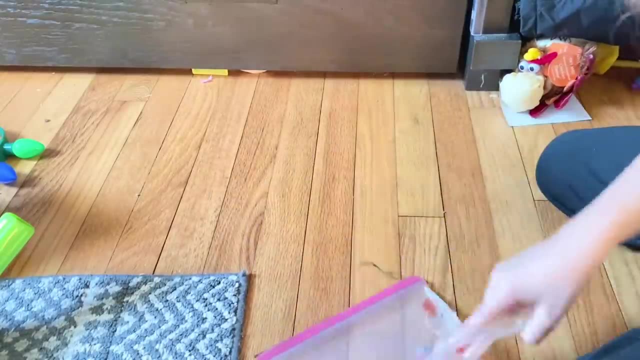 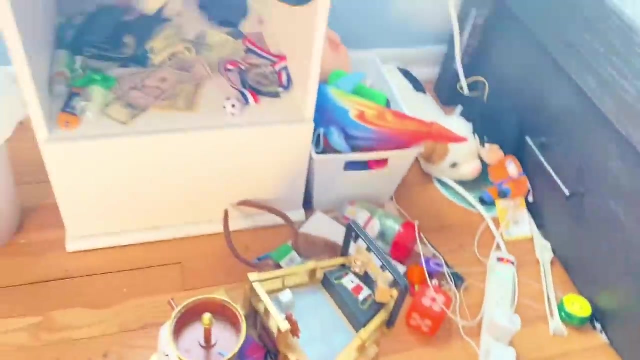 holding on to so much stuff and not knowing how to let it go. Our self-worth is not determined by all the stuff that we have and how it makes us feel, Because I know firsthand how stuff can make you feel safe and secure and abundant and joyful. And you just pour. 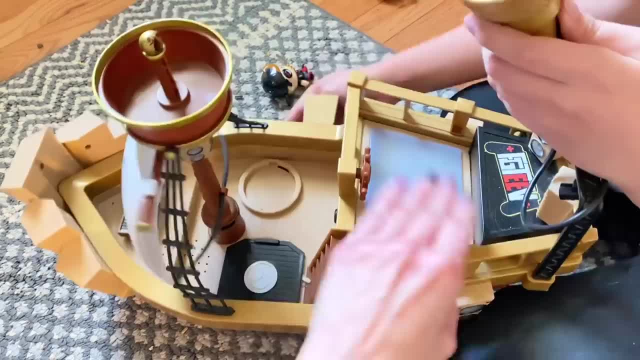 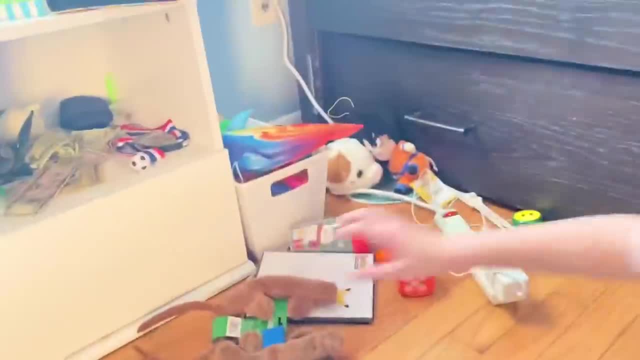 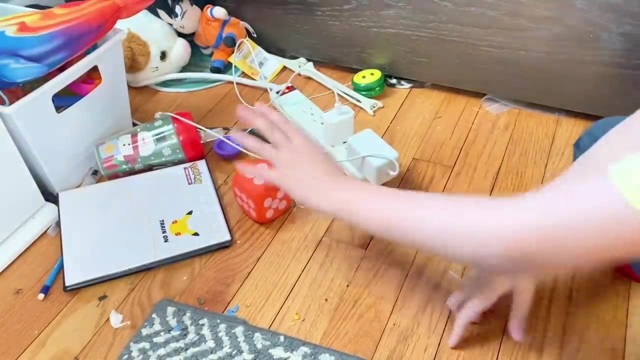 all of your emotions into these items that aren't even real. We attach those emotions to these items, not the items itself. The items aren't jumping up and giving me a big hug. I humanized all of my toys as a kid and it carried into adulthood, And that's what I'm trying to do. 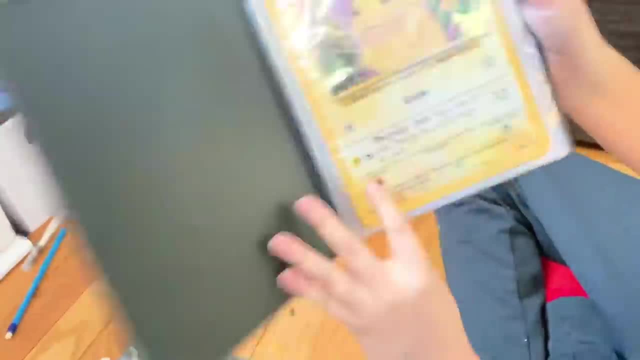 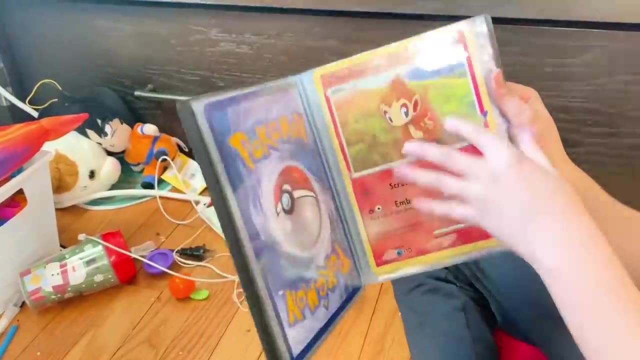 with all of my things, And we actually did that, And so I give my kids a lot of praise because they already know that they can have it and they already know what they can be posted on. This is a great way to break that generational behavior. It ends here, My children, 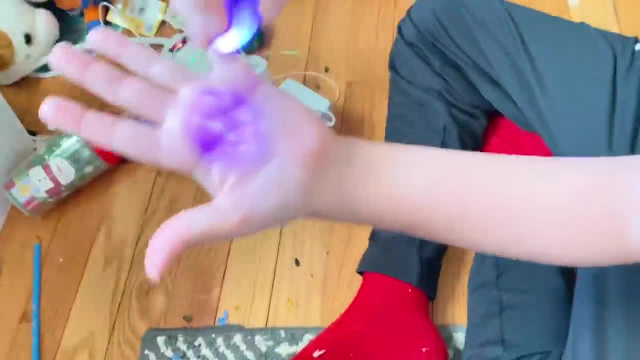 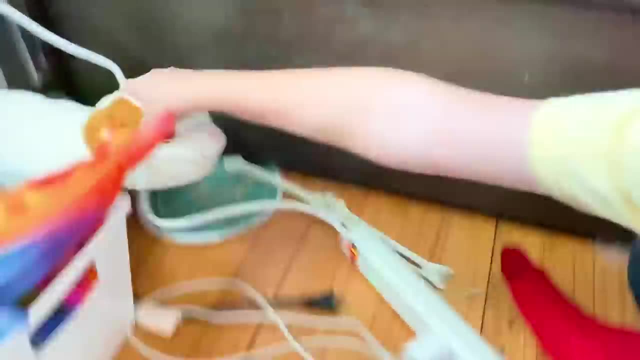 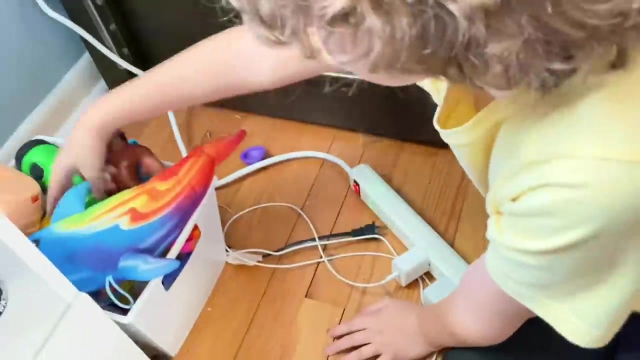 will not struggle with hoarding behaviors because they'll already know the love of having an open space, being able to distinguish what pieces they do love and what pieces they don't love, and just develop these decluttering muscles- My generation- that they'll already know how to modify these behaviors so that it doesn't develop into a 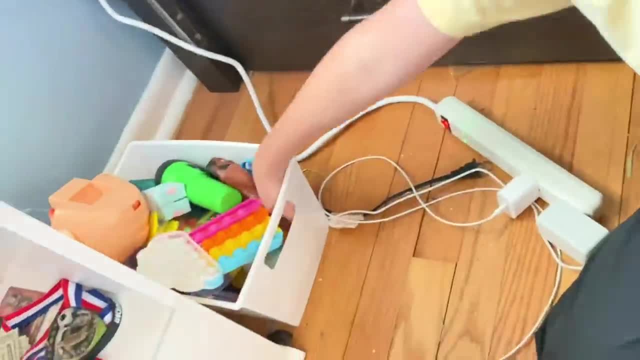 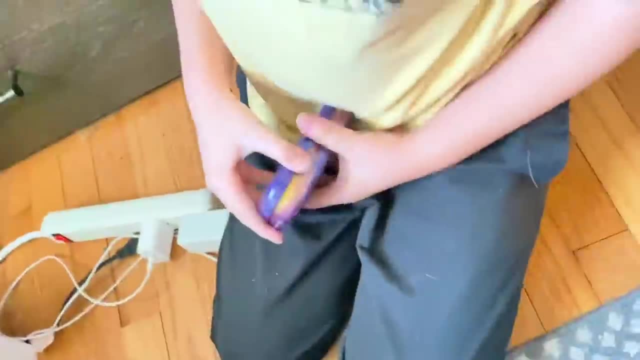 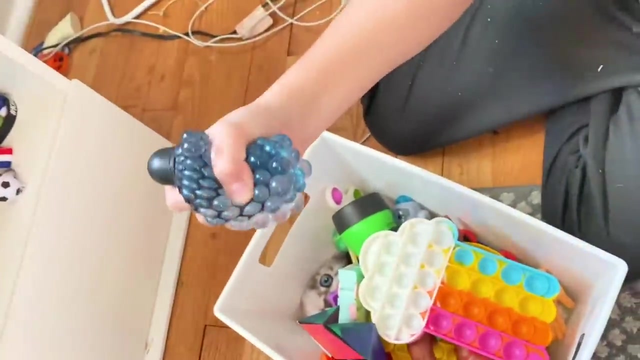 full-blown level five hoarding situation, Because I had reached and crossed over to a level four hoarding at my worst point because I had blocked doorways and unusable bathrooms because it was filled to the brim with stuff. And it's been a long yet wonderful healing journey. I just want. 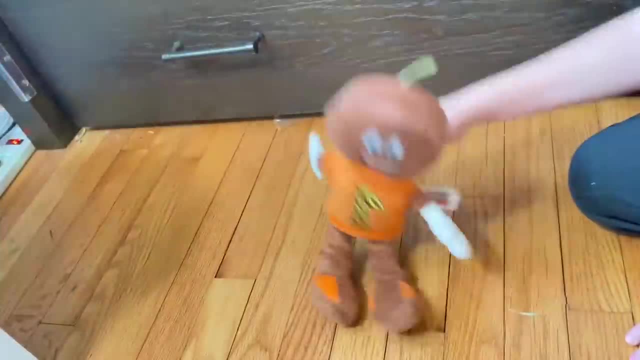 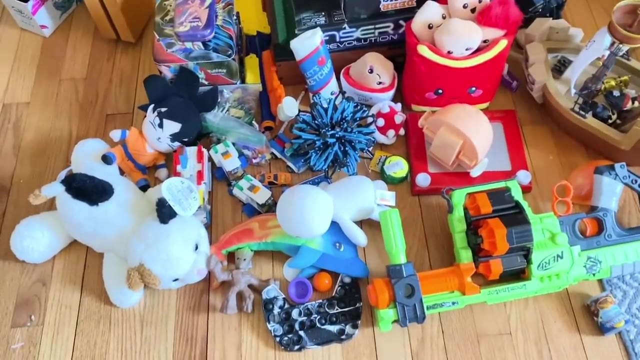 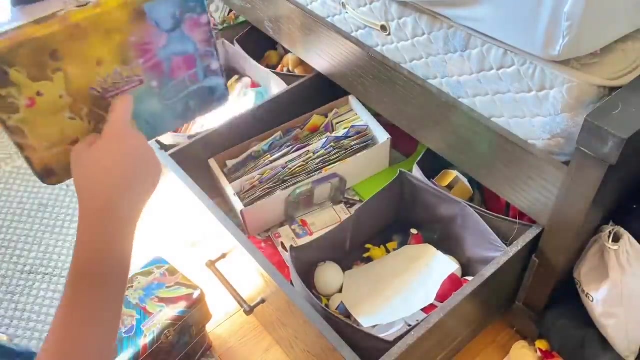 my children to experience the freedom of not being held back by their things. And this is Tyler's keep pile. This is what he wanted to keep in his room, And again, I didn't make any decisions for him. I let him take the lead on this. So what's important is if we're going to keep all these fun. 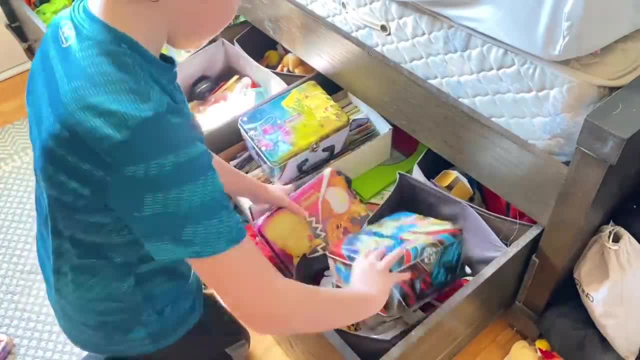 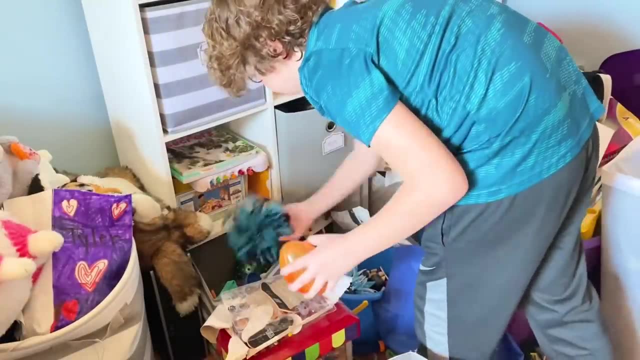 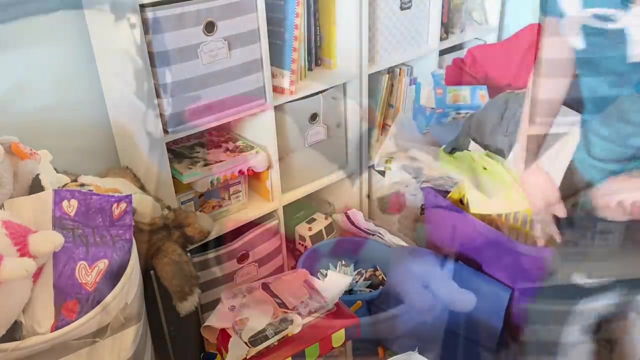 things, then we have to put them back where they belong. We have to create these designated homes where all the items are. That way we can see what we have all together, And if a home is packed to the brim because it's overflowing with stuff, then we can make the decision of what can we let go of and what do. 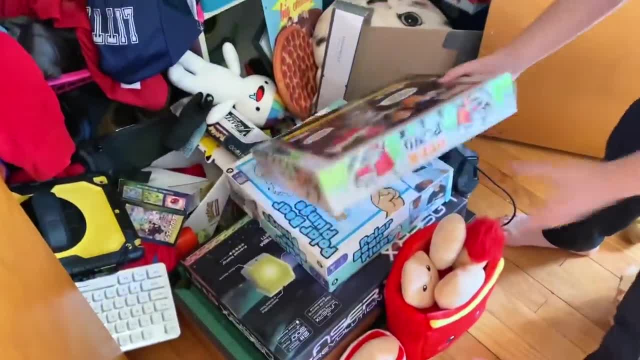 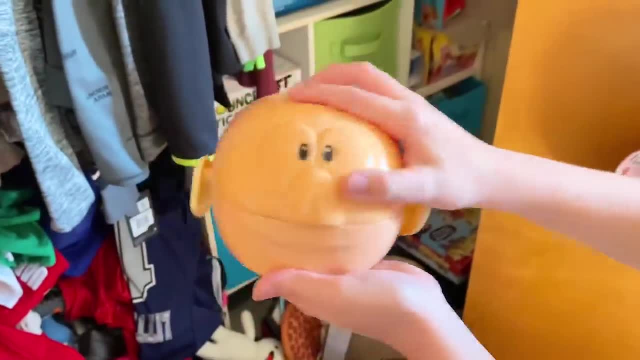 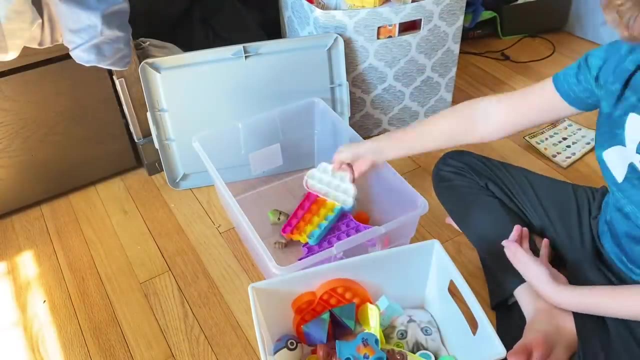 we want to keep based on that category. These are skills that I did not learn, but I'm so happy that I'm able to teach my children because I feel like I'm coming full circle in my recovery, And one of Tyler's favorite things to play with would be all of his fidget toys. So that's why we're transferring all. 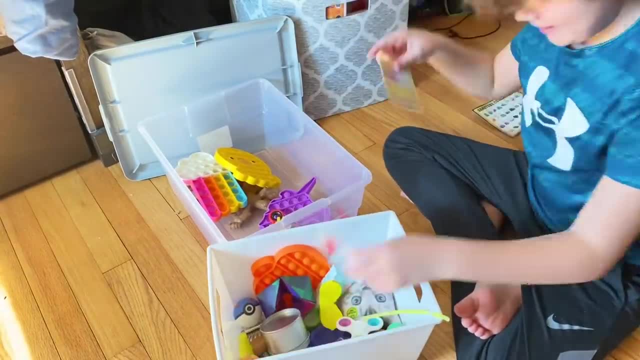 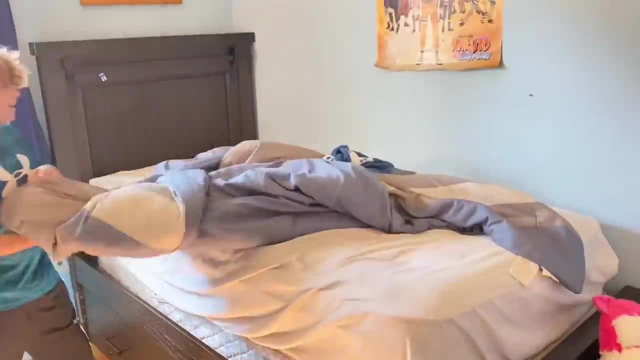 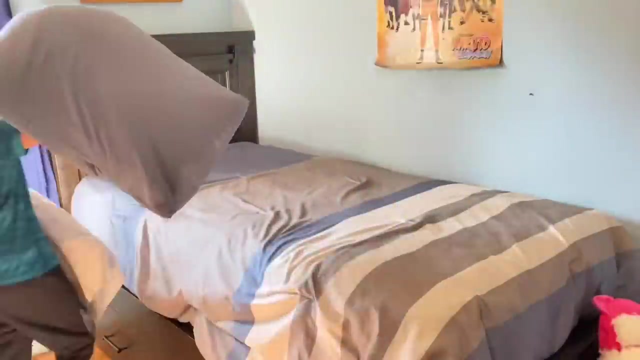 his favorite fidget toys into this bigger container. so it's all together. And then I had Tyler make his bed, because the room really does feel so much cleaner and tidier when the bed is made And, honestly, probably since high school till maybe, like when we redid our bedroom. 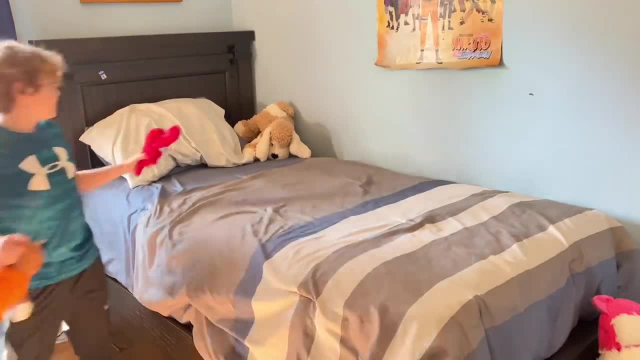 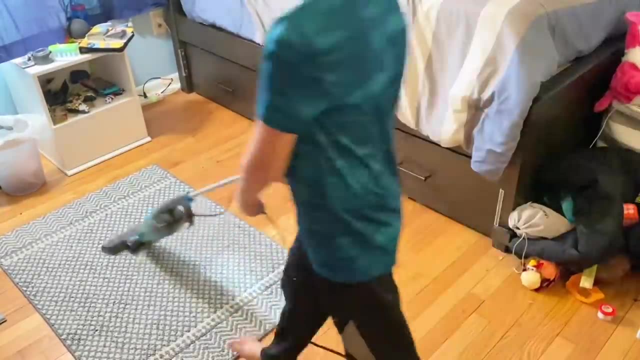 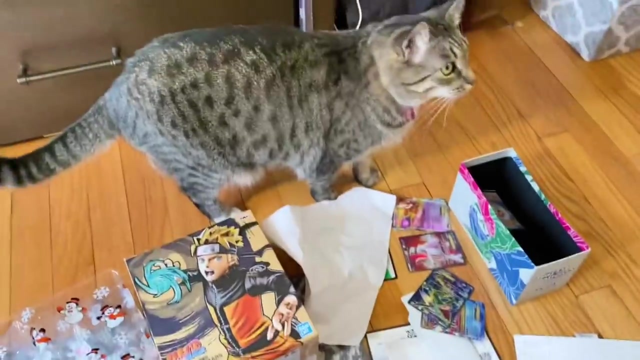 I never made the bed, And when I saw just how nice the room looked with a made bed, that's when I started to change that habit. And now Pepper, our decluttering manager, is very happy to show you Tyler's Tossy, Tossy pile. I let him make the decisions. 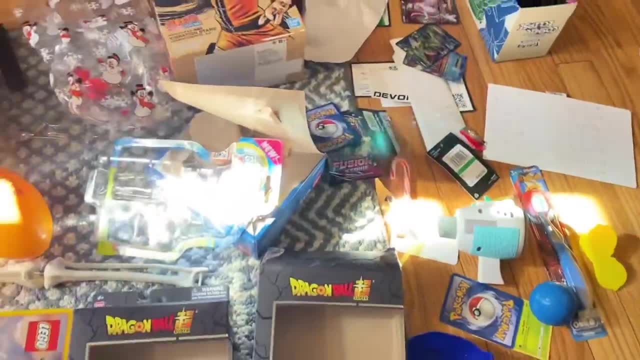 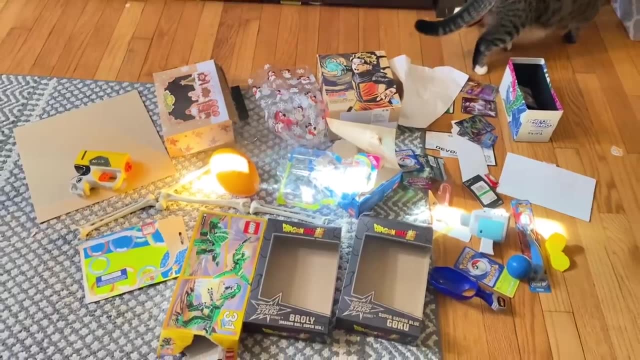 on what he was going to let go of. I didn't encourage him to keep anything, And I also didn't encourage him to keep anything, And I also didn't encourage him to keep anything. I didn't encourage him to let go of anything. This was all his decisions And, of course, 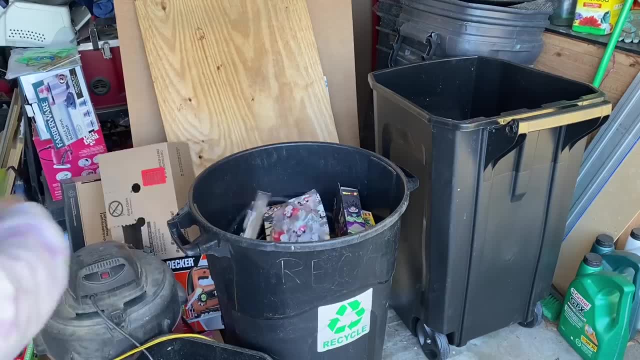 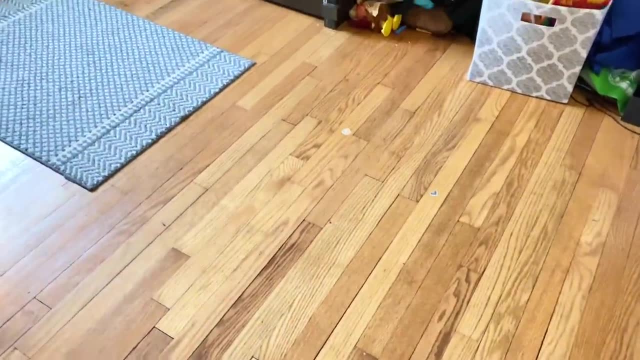 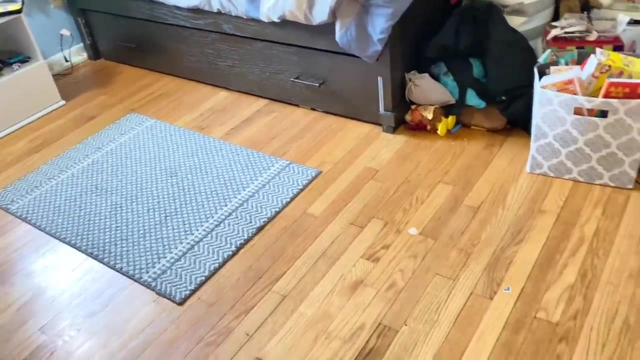 we're going to recycle as much as we can, because it's very important to my heart that we do our best to keep things out of a landfill, And I'm so happy to show you what Tyler decluttered and cleaned up today. He focused on this area right here in the middle of the room in front of his 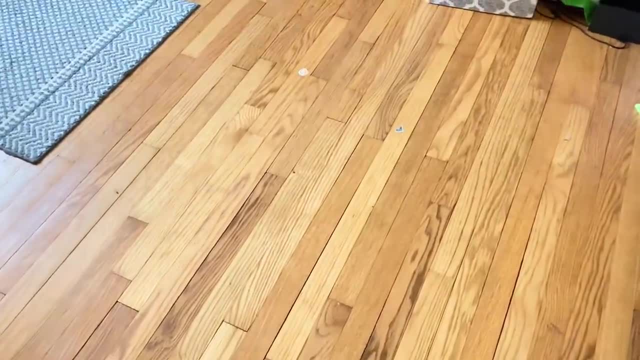 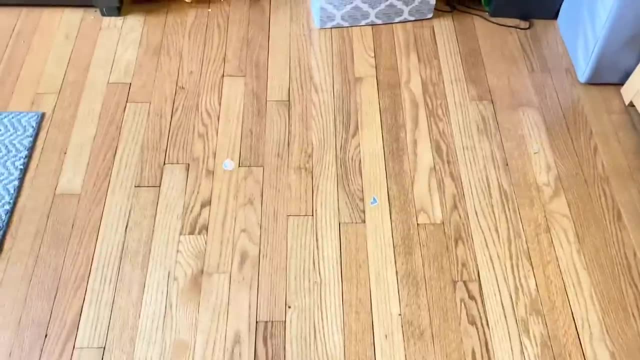 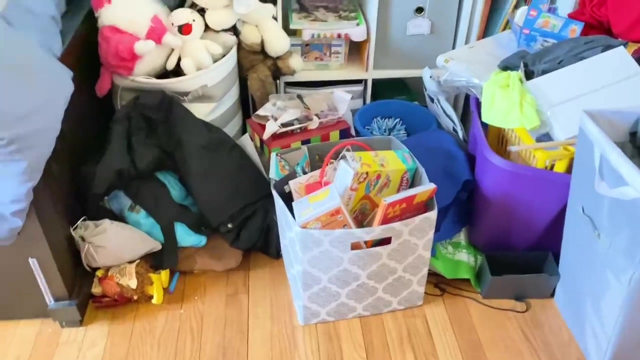 bed. Again, this was his decision And I let him declutter until he felt good And said that he was done for the day. We're trying to make this a positive experience where he feels empowered in his room and that he wants to continue to tidy up his room.